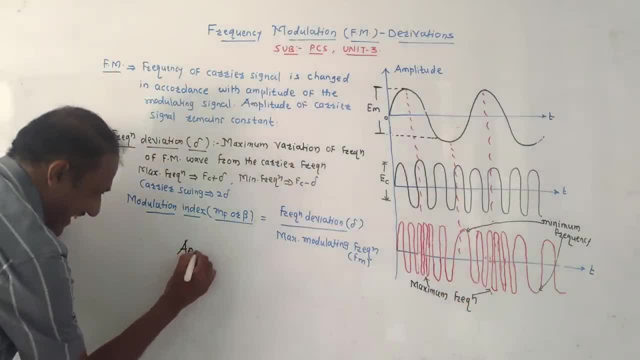 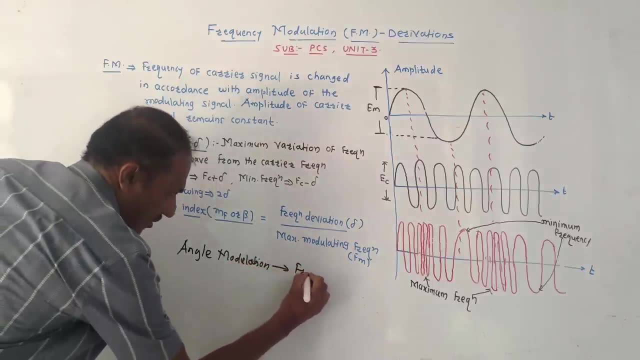 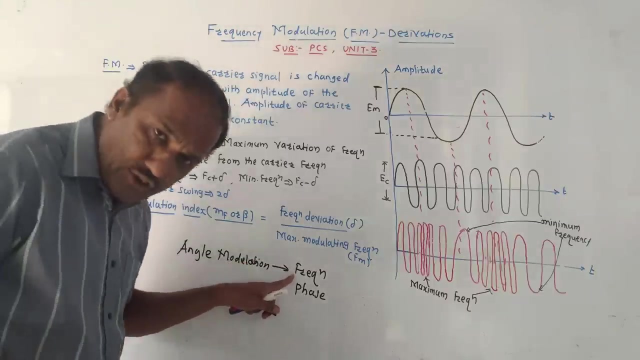 Actually there is one common term which is known as Angle Modulation. So in case of Angle Modulation, either frequency of carrier signal is changed or phase of carrier signal is changed. If the frequency of carrier signal is changed with respect to the modulating signal, 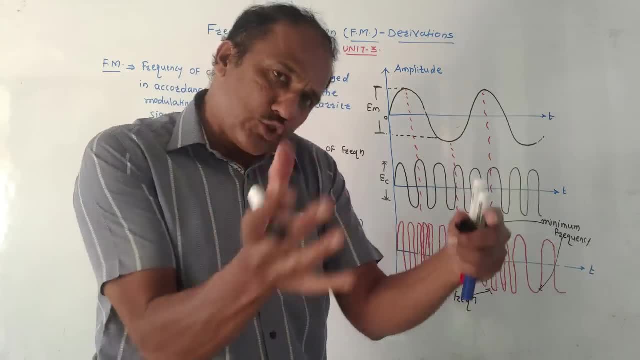 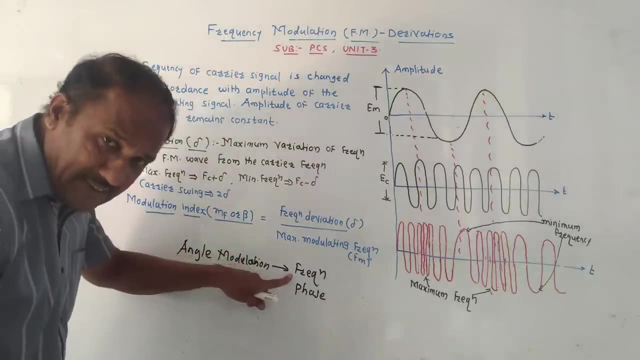 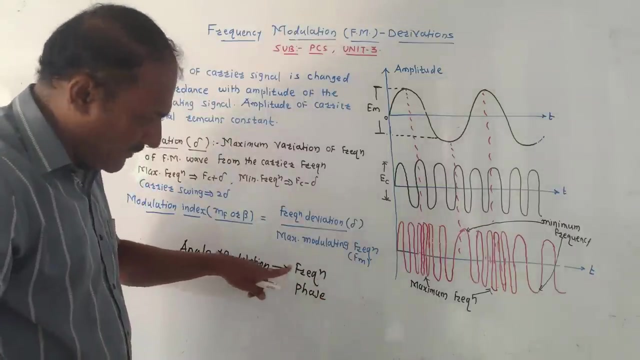 we know that modulating signal is an information signal which is superimposed with some carrier signal and carrier signal is a high frequency signal. So if frequency of the carrier signal is changed according to the modulating signal, then it is called Frequency Modulation. 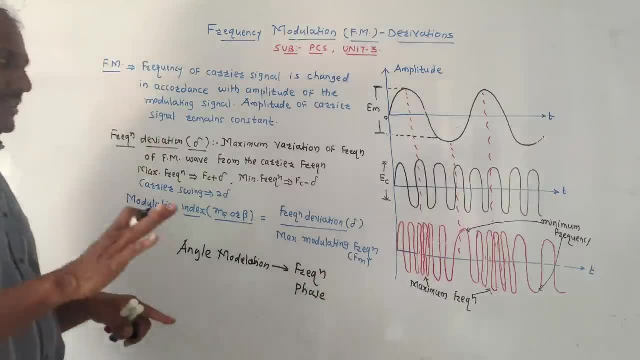 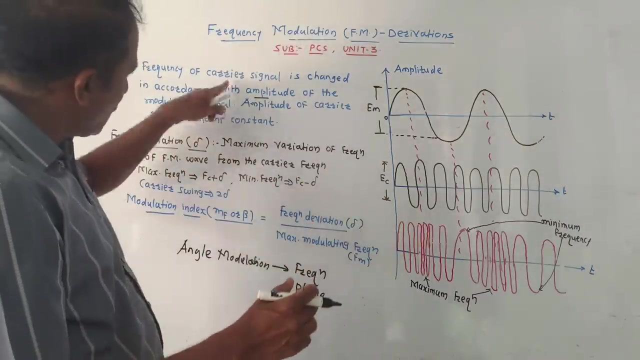 On the contrary, if phase is changed, it is called Phase Modulation. Now first part, definition of FM. Frequency of carrier signal is changed in accordance with amplitude of the modulating signal. If the frequency of carrier signal is changed with respect to the amplitude, then it is called Frequency Modulation. 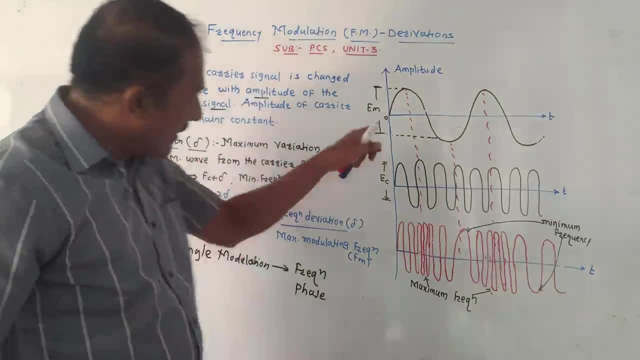 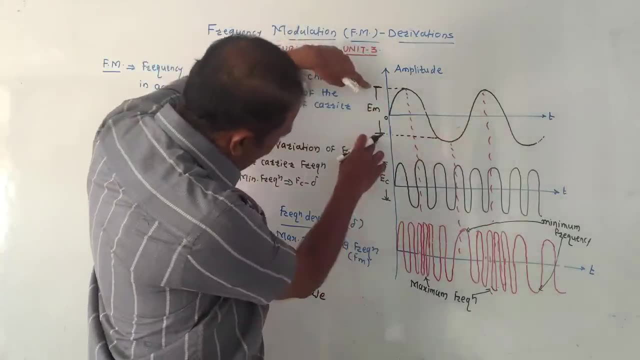 Whereas amplitude of the carrier signal remains constant. Now refer this diagram. In this diagram, the first diagram is of modulating signal, ie of information. Its amplitude is denoted by E M Maximum Amplitude. Now this is the second diagram. 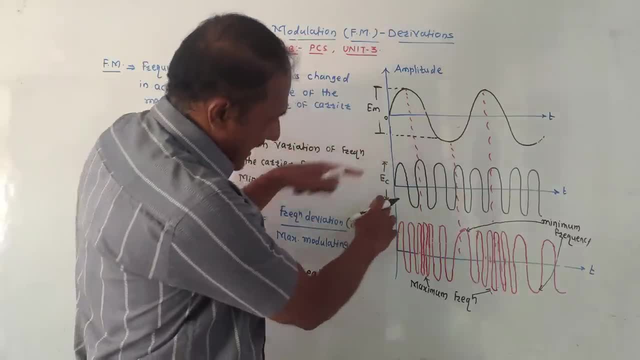 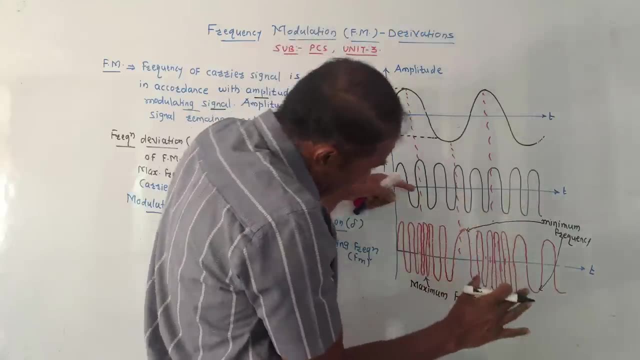 This diagram is for carrier signal. Its amplitude is E C. Presently, the amplitude of the carrier signal is constant and the frequency is also constant. Don't doubt, we are marking the time on this axis. Now look. what does frequency modulation mean? 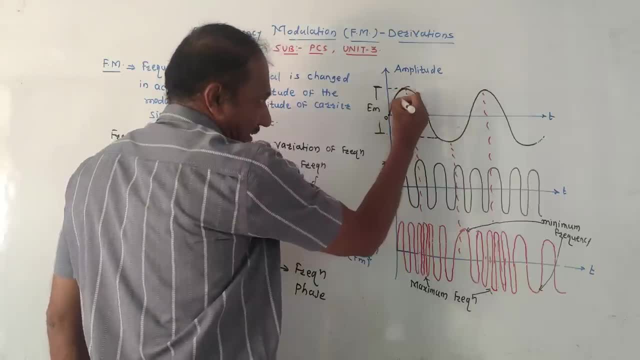 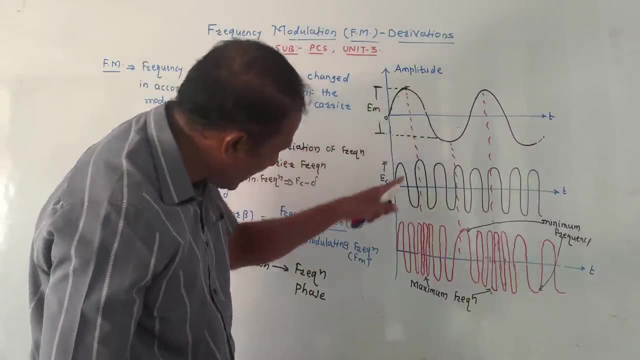 From here the positive cycle is starting. Modulating signal ie, information signal, is getting maximum value here. With respect to this, as the amplitude of the modulating signal changes, the frequency of the carrier changes, Amplitude remains constant. 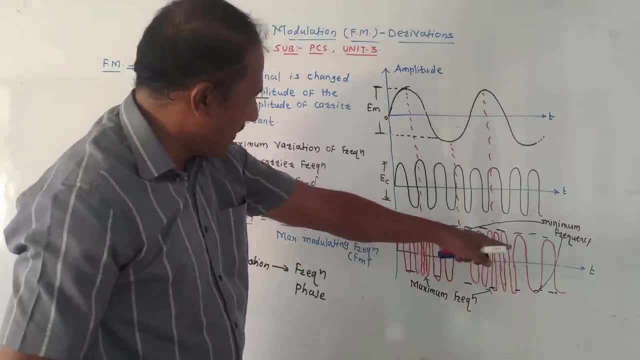 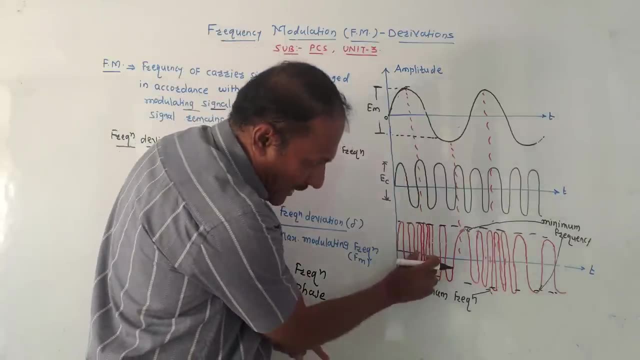 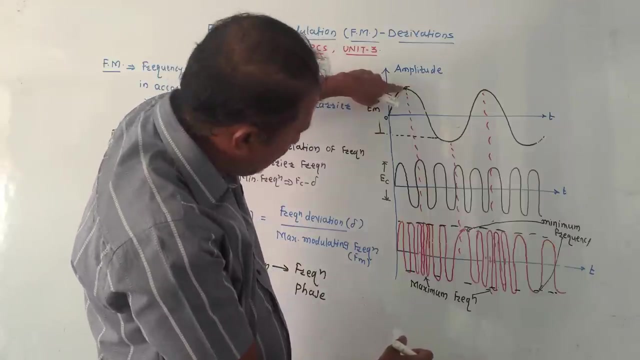 Look, the amplitude is constant. Now, as the amplitude increases, the frequency increases. The gap is less and, with respect to time, the frequency increases. So at this point, where the amplitude of the modulating signal is maximum, you are getting maximum frequency. 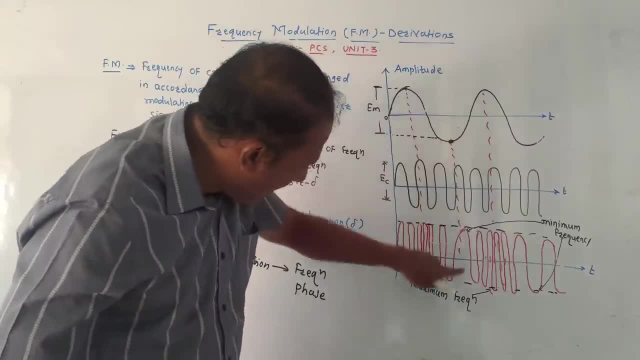 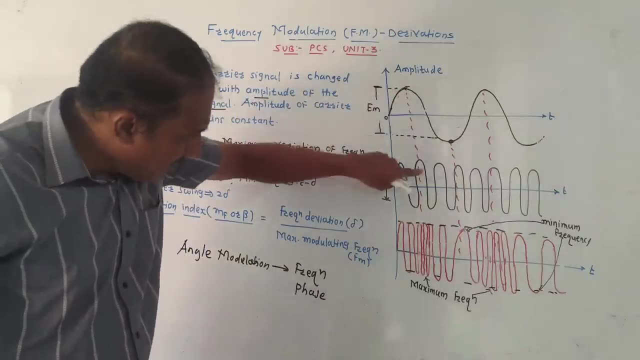 Here the amplitude of the modulating signal is less, it is minimum. So here the minimum frequency will come. Likewise, in accordance with the amplitude of the modulating signal, the frequency of the carrier wave is changed. This is called frequency modulation- FM. 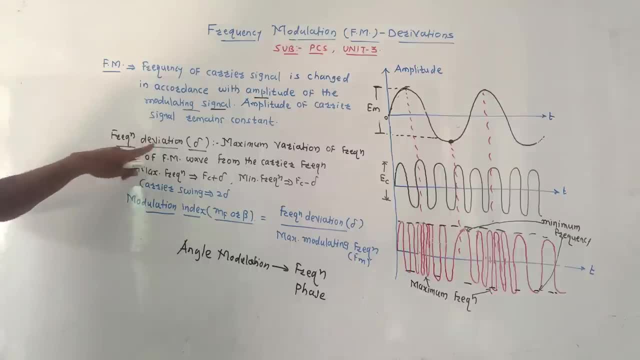 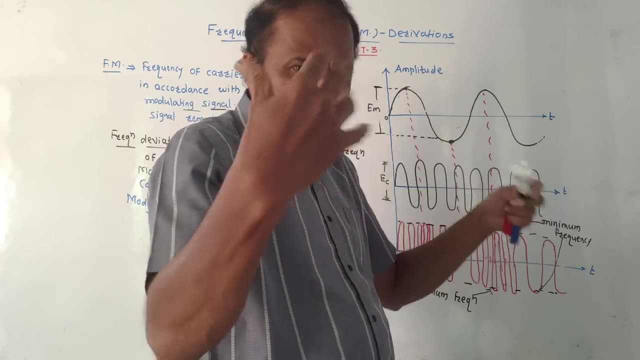 Now some important terms related to FM. First is frequency deviation. Now look how to remember. Deviation means how much change is happening with respect to the standard value. For example, if you have a circuit whose voltage is 5 volts. 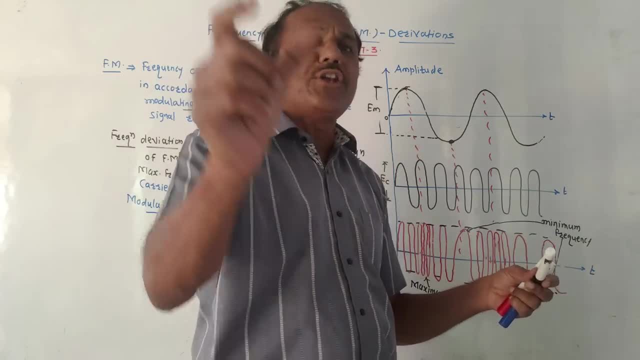 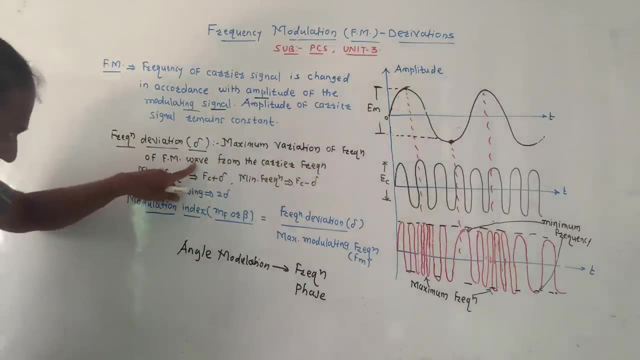 and practically reading, is 5.1, then the deviation will be 0.1, like this. So frequency deviation is denoted by delta. The maximum variation of frequency of FM wave from the carrier frequency, That is, the carrier frequency, will be denoted by fc. 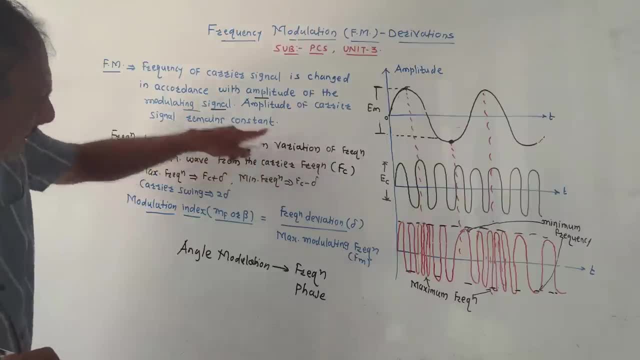 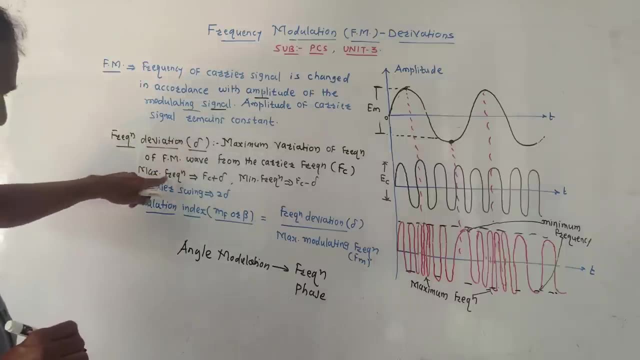 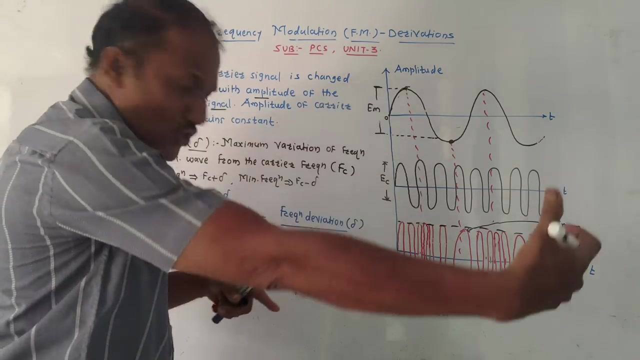 With respect to this carrier frequency, how much deviation, how much change is happening in the frequency of FM wave? this will be called frequency deviation. Now, maximum frequency that is denoted by fc plus delta, Because the carrier frequency is changing. delta means how much change is happening. 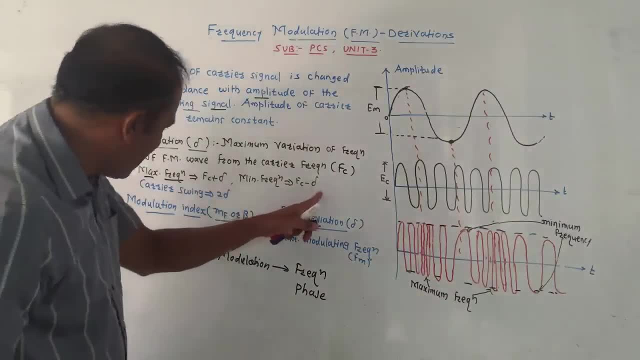 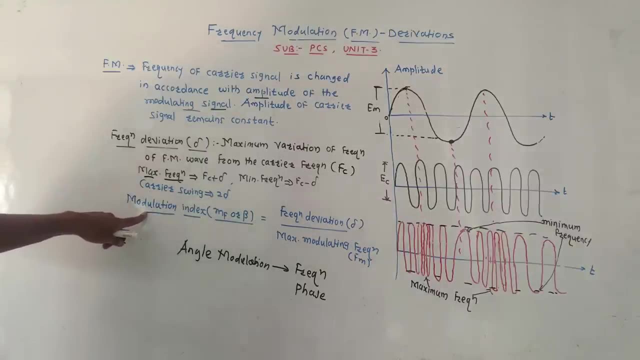 So maximum will be fc plus delta, Minimum will be fc minus delta. The two-delta amount is called carrier swing. The next parameter is modulation index. It is denoted by m to the base f because it is for FM modulation or beta. 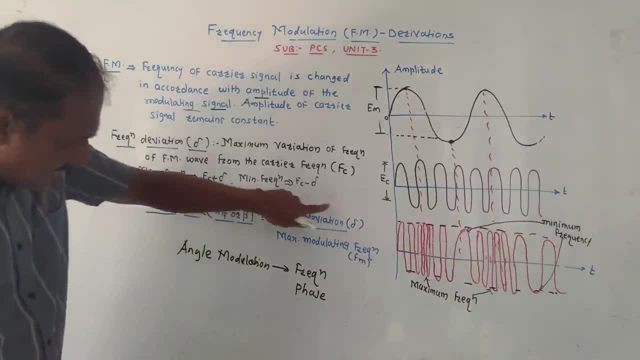 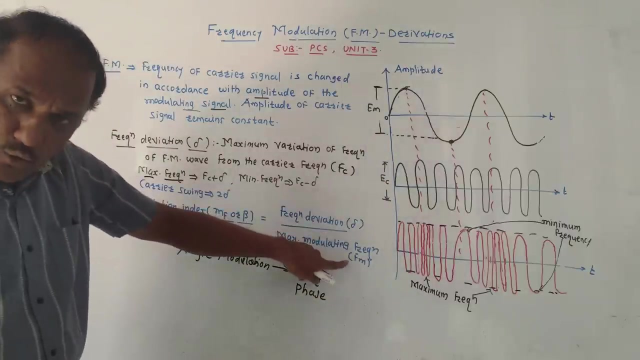 One more notation is there. It is the ratio of frequency deviation to the maximum modulating frequency. It is fm. Note down: fc is carrier frequency Modulating signal. its frequency is fm. So it is ratio of frequency deviation that is delta to the fm. 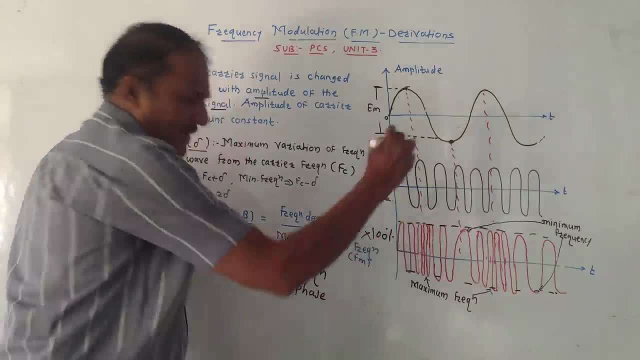 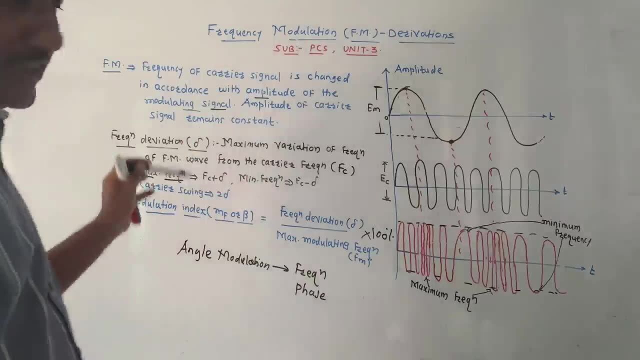 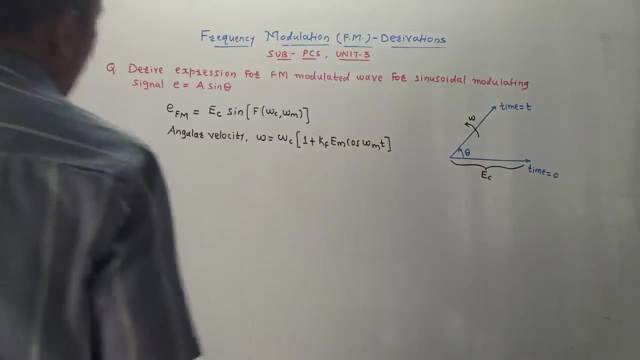 This is the ratio, So it is usually expressed in terms of percentage. So multiply by 100.. So these are the few basic terms related to the frequency modulation. Now let us derive the equation for FM wave. Now let us derive the expression for FM wave. 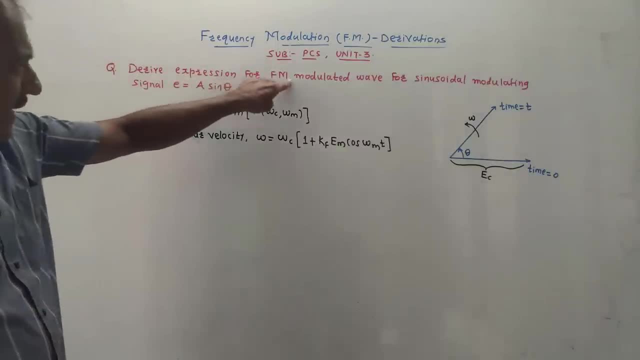 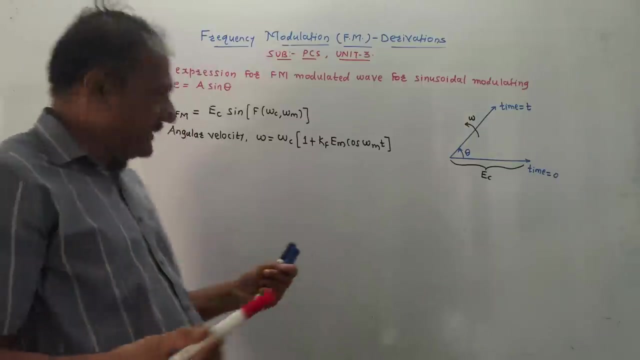 The usual question is: derive expression for FM modulated wave, for sinusoidally modulating signal, E is equal to A sine theta. A is amplitude Notation can be anything Okay Here. given equation is in terms of theta. Now you need to remember some basic things. 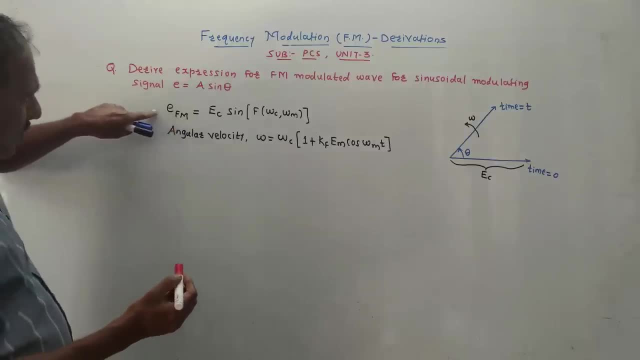 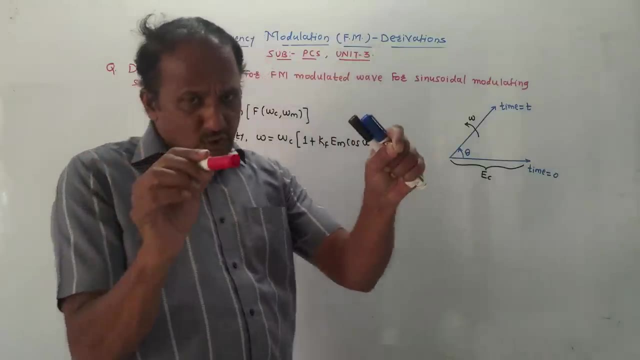 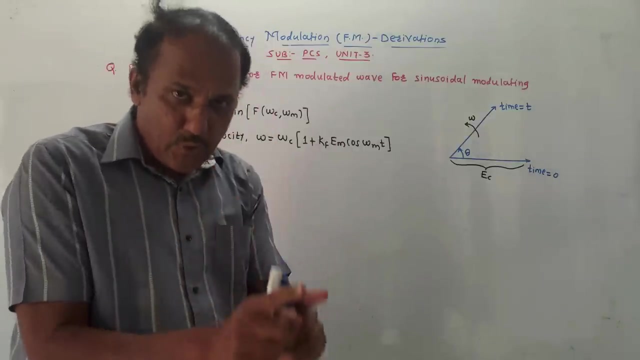 EFM is the equation of FM. wave is equal to EC. EC is the amplitude of carrier wave. Note that in case of frequency modulation, frequency of the carrier wave is changing, Whereas amplitude and phase of carrier remains same, only frequency is changing. 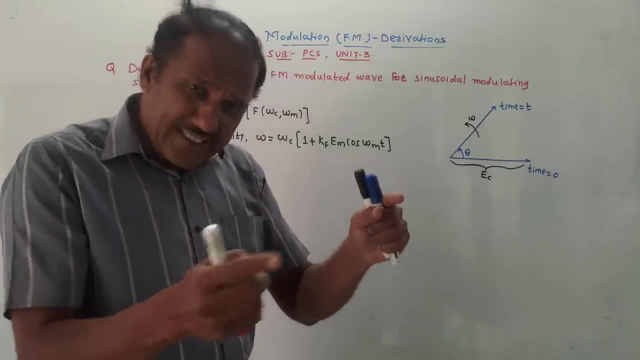 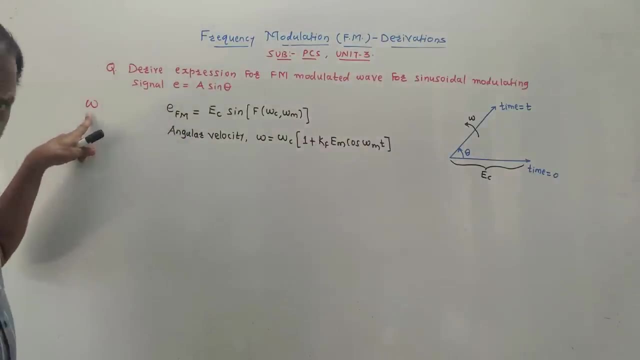 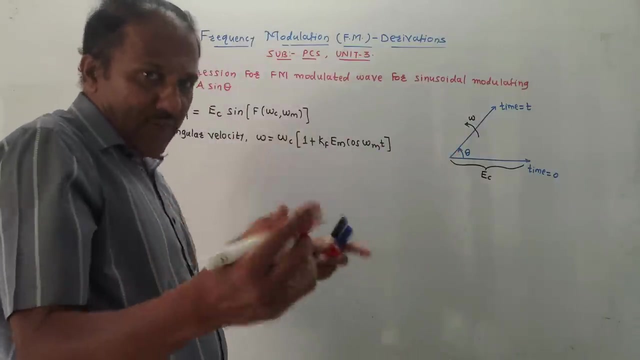 Now, since frequency is changing, there is some velocity. That velocity is called angular velocity, denoted by omega. Don't get confused. as far as notations are concerned, Omega is the angular velocity with which the FM wave is changing, Whereas 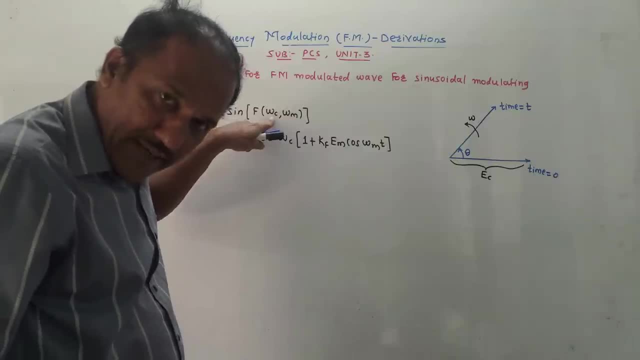 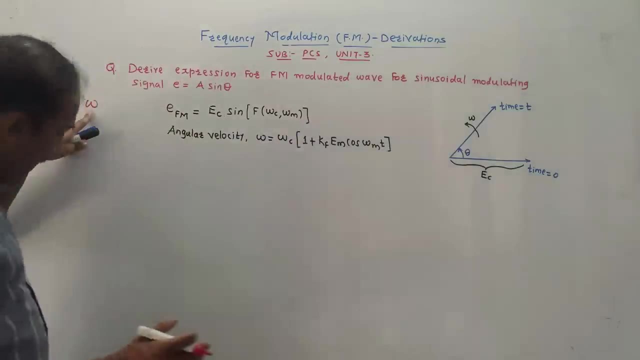 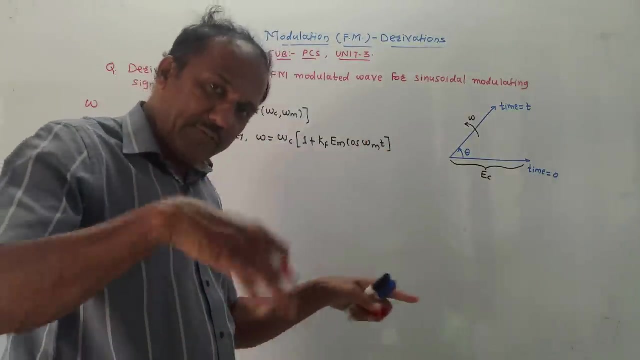 omega C is the frequency of carrier wave, angular frequency of carrier wave. Omega M is the angular frequency of modulating signal. So angular velocity is function of omega C and omega M. That is, it is function of carrier frequency and modulating frequency. 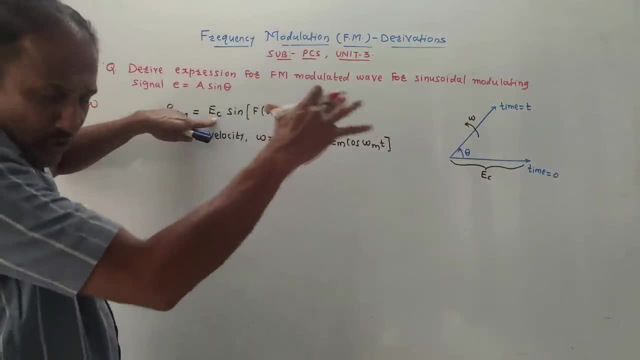 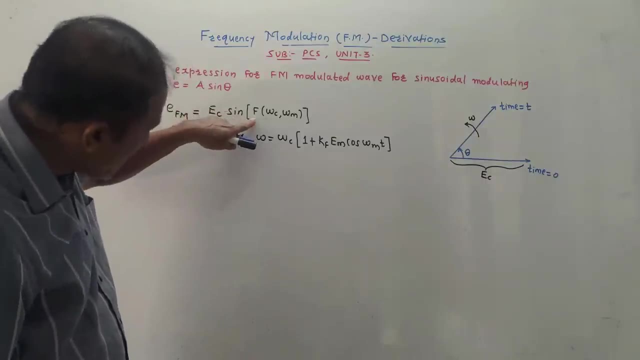 So general expression. I have written it like this EC, because its amplitude of carrier wave remains same, So its amplitude is written as EC, Sine We have assumed sinusoidal nature And function of F means function of 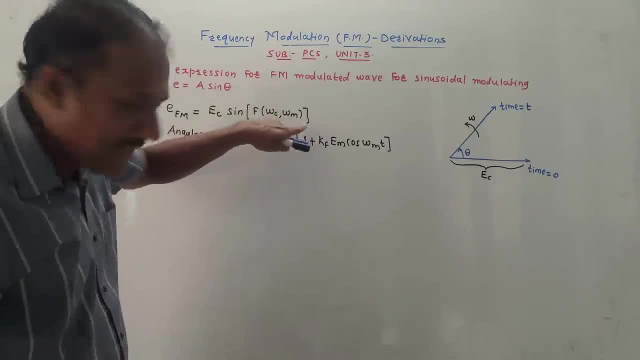 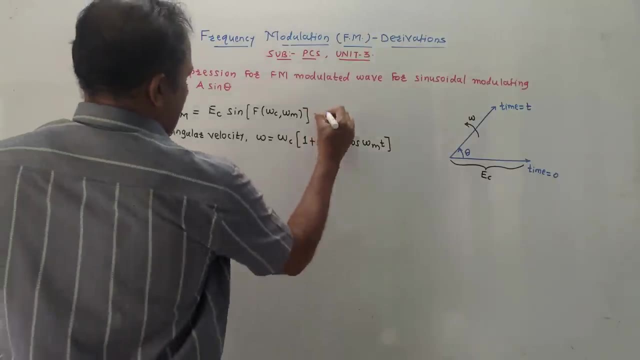 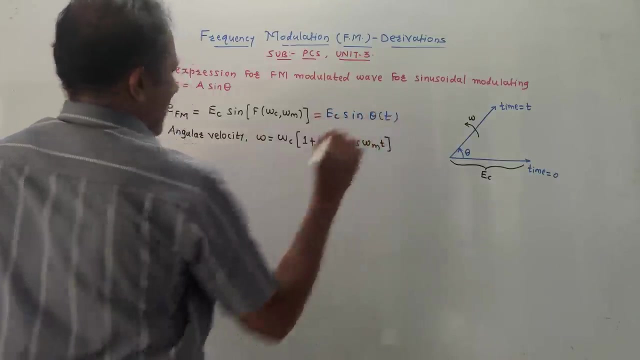 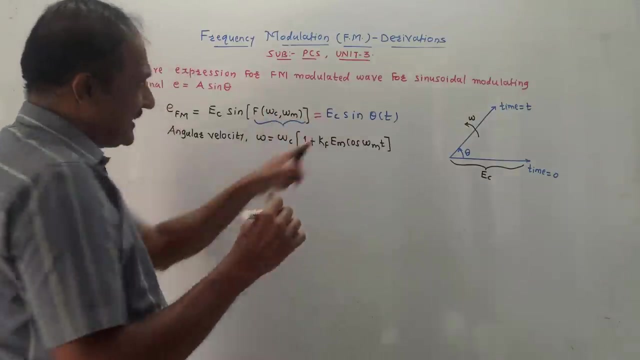 omega C. omega M means function of omega C and omega M. Same expression. this expression, I can well write it as EC sine of theta T, Where theta T means function of omega C and omega M. This term, I have replaced it by theta T. 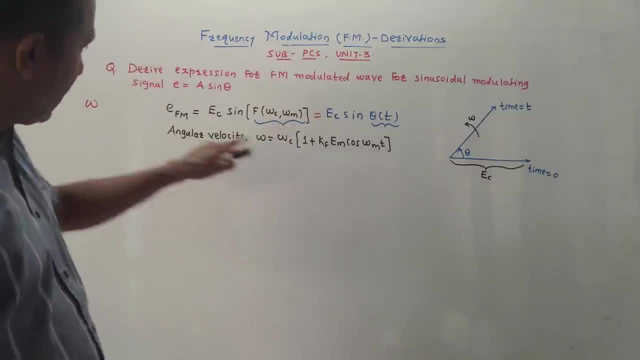 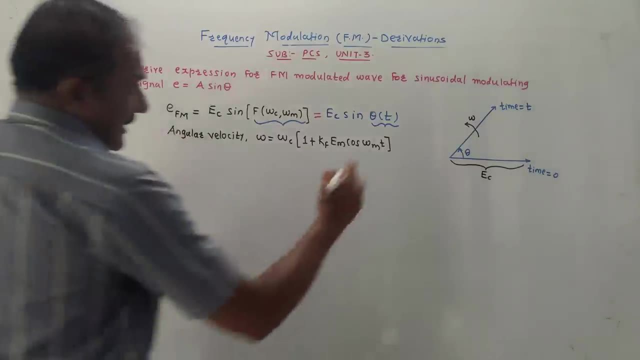 Where theta T means function of omega C and omega M. This is the generalized expression of FM wave. Now you need to remember only one equation. Let us say this is equation number 1.. This is equation number 2.. I will explain what is this. 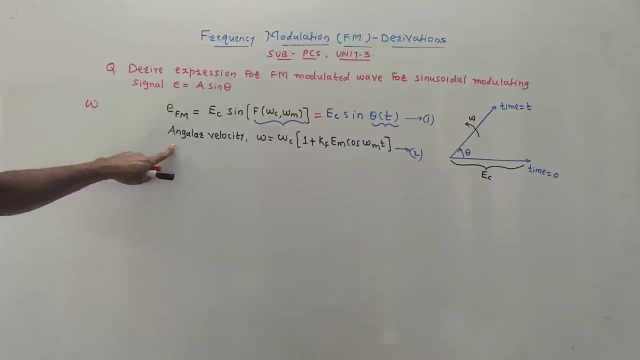 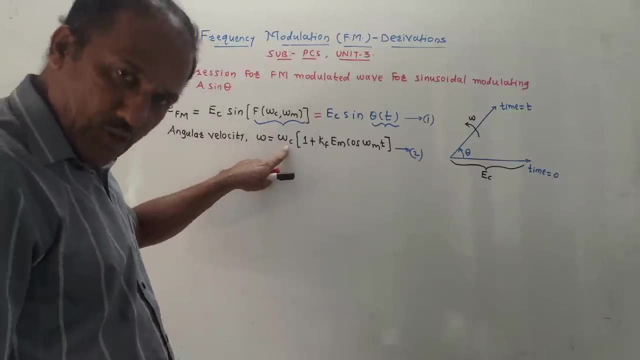 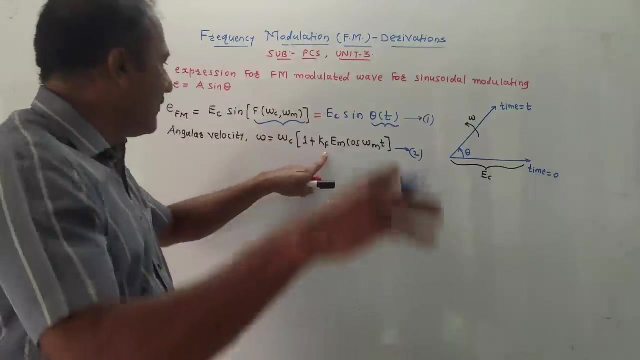 You need to remember only one equation to complete this derivation. The angular velocity omega for FM wave is given by omega C. Omega C is the frequency of carrier wave, carrier signal One plus KF. KF is some constant term. Since it is related to FM wave, it is denoted by KF. 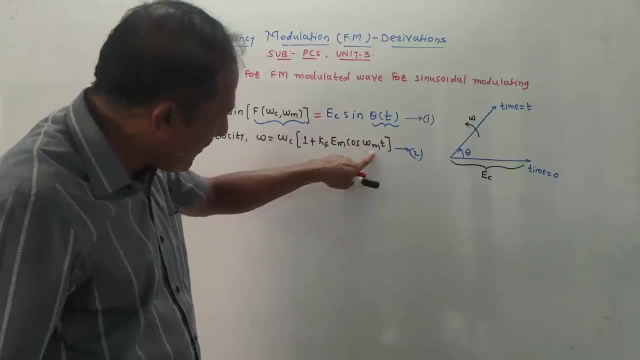 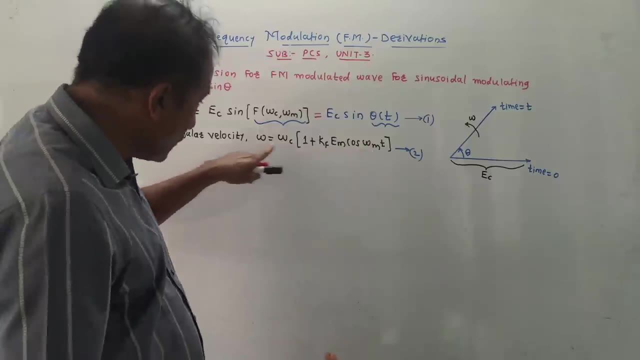 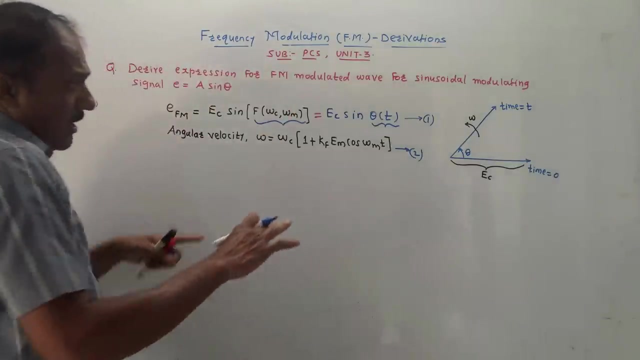 EM. EM is the amplitude of modulating signal: Cos, omega, MT. So for the simplicity, we have assumed cosine wave for the modulating signal. So this is the expression for angular velocity of FM wave. You need to remember this equation. 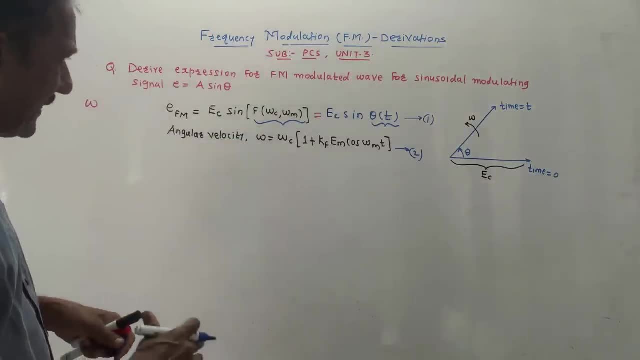 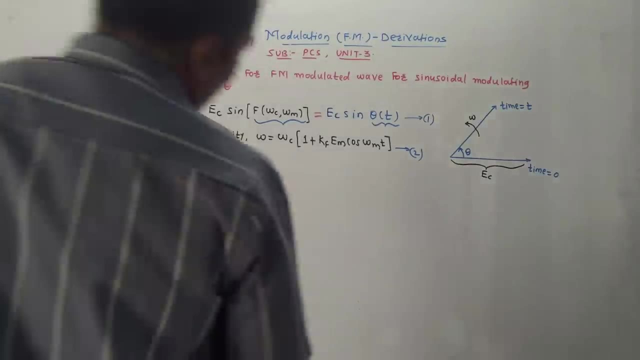 So this is the expression for omega. Now next part is: since we have got this expression, we will derive the complete thing related to FM wave. Now see how to correlate. I have made a diagram Here. it is written: EC. 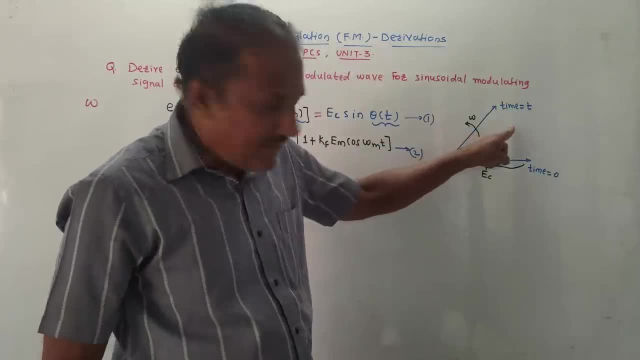 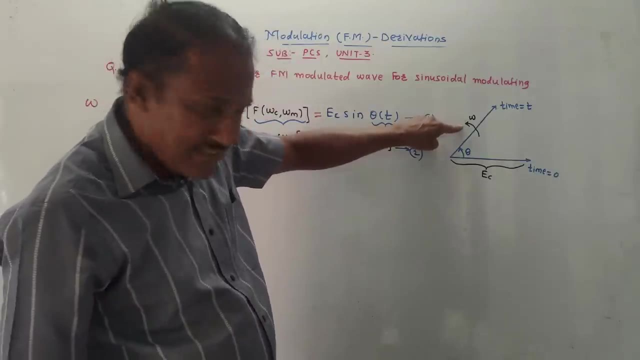 On this axis, time T is equal to 0.. On the other axis, I have written time T is equal to T. T is some value of time period. This angle is written as theta. Omega is the angular velocity. This means that EC is a vector which is rotating with the velocity omega. 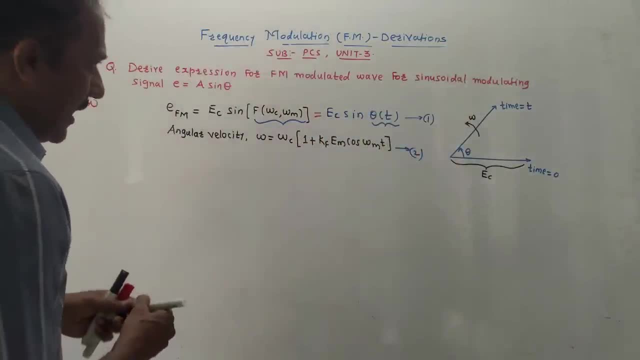 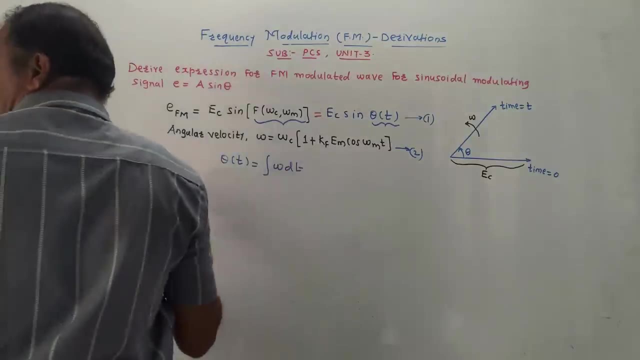 Make the thing simple, Remember this: If I have to calculate theta T, it is obtained by integrating omega. So theta T can be obtained by integrating omega. Naturally, variable of integration will be T. So let us put this value. 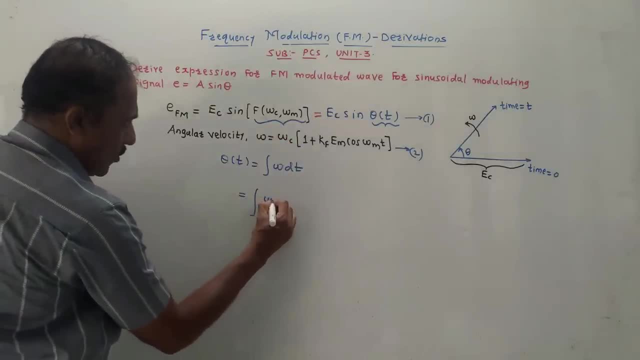 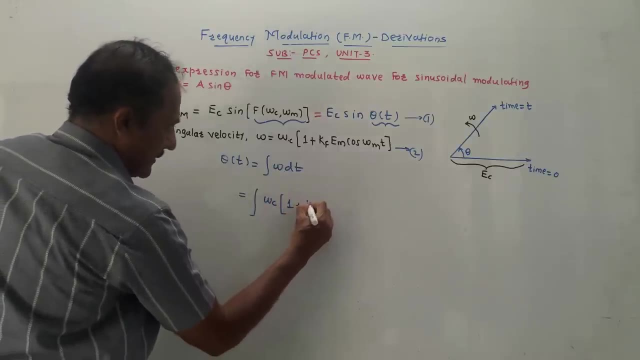 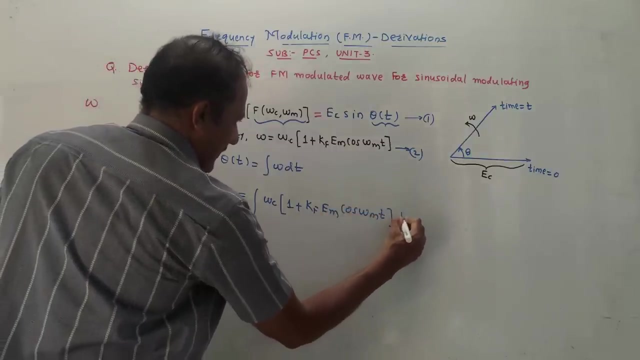 So I can write it like this: Integration, omega C. I am putting value of omega, That is equation 2, over here. So omega C in the bracket 1, plus KF, EM, cos, omega, Cos, omega, MT. The variable of integration is DT. 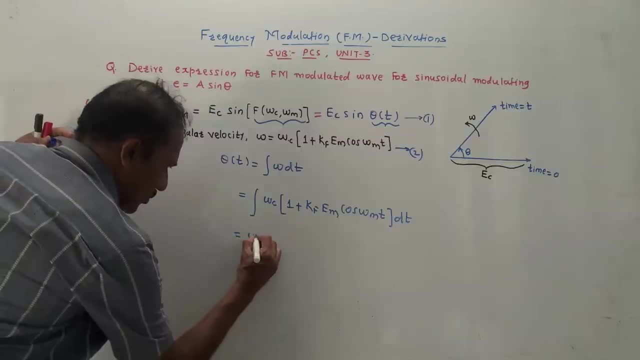 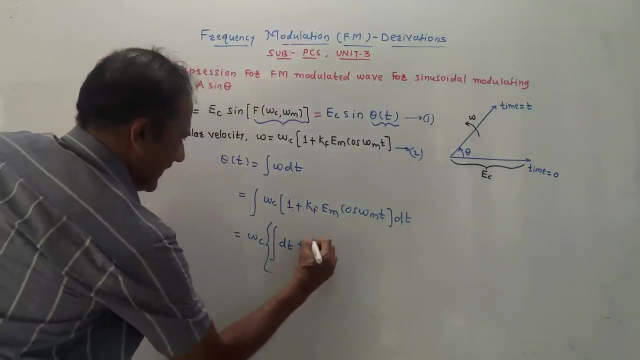 Omega C is constant. It can be taken outside the integration. So omega C integration. Different terms are written. It is DT 1 into DT. Let us make another bracket: 1 into DT is DT Plus second integration. This is one integration. 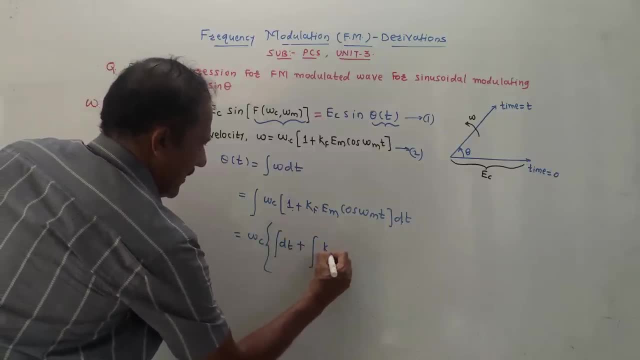 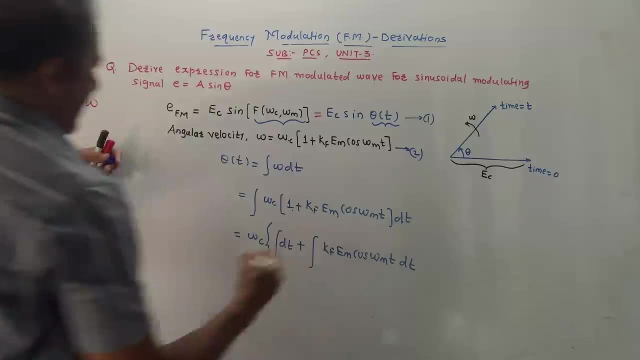 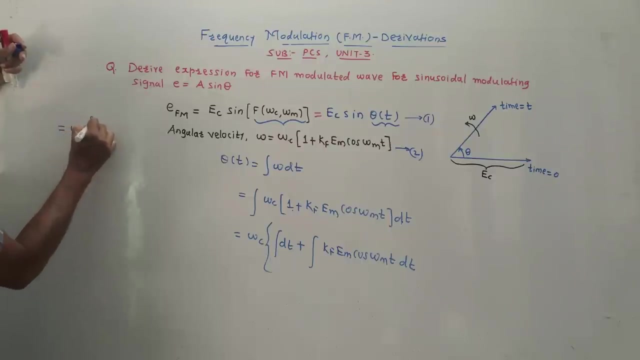 Integration DT. Second integration: KF, EM, cos, omega MT, DT. Now we have to solve this integration. So omega C is outside As it is. it will remain. This bracket is till here. First integration of DT will come. 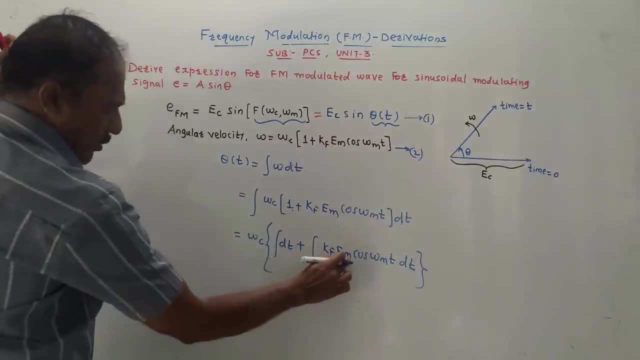 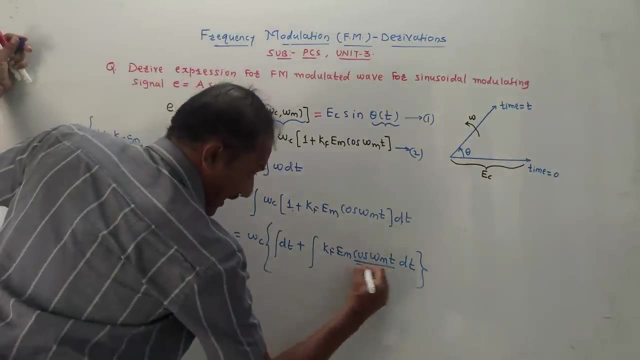 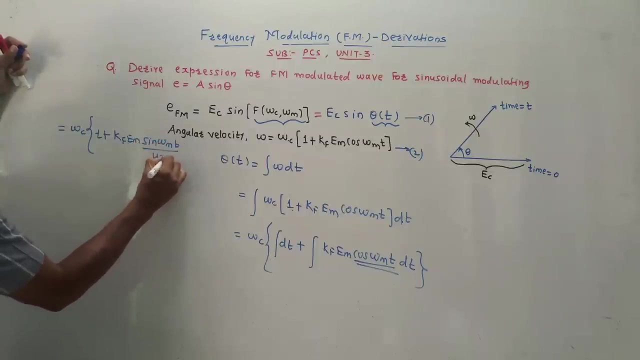 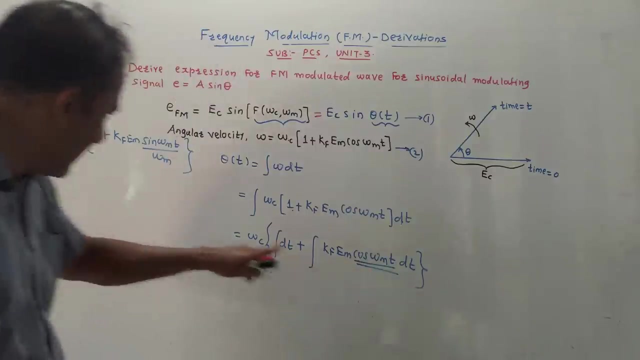 T plus KF EM is constant, So I will be writing it as it is: KF EM. sin Cos omega MT. integration is sin omega MT Divided by omega M. This is integration of cos omega MT, KF EM as it is. 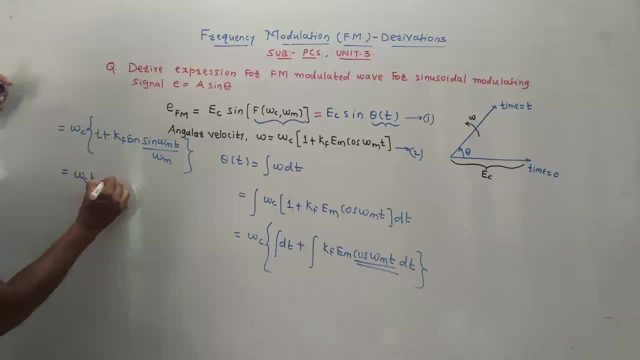 So it can be written as omega CT Plus omega C, KF, EM, sin, omega T, Sin omega MT Upon omega M. We know that Basic equation of omega is 2 pi F, So I can well write this first term. 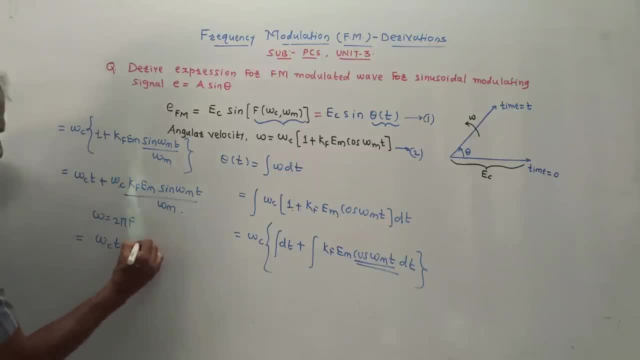 I will keep it as it is Omega CT plus Here. Here I write 2 pi FC This in place of omega C. I will use other color For this omega C. I have written 2 pi FC Similarly for this omega M. 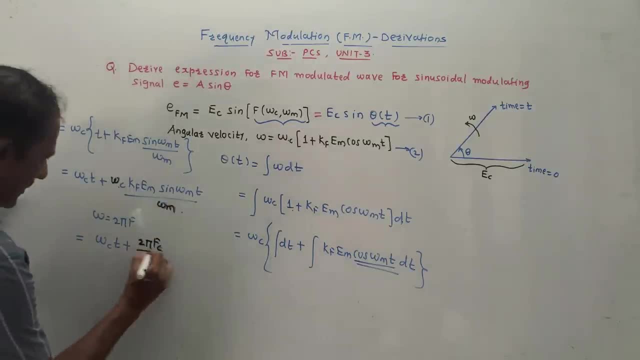 I will be writing 2 pi FM. So here I write 2 pi FM. Rest of the terms will be as it is. So it is KF, EM, sin omega, MT. Now these two terms are cancelled. So it is FC upon FM. 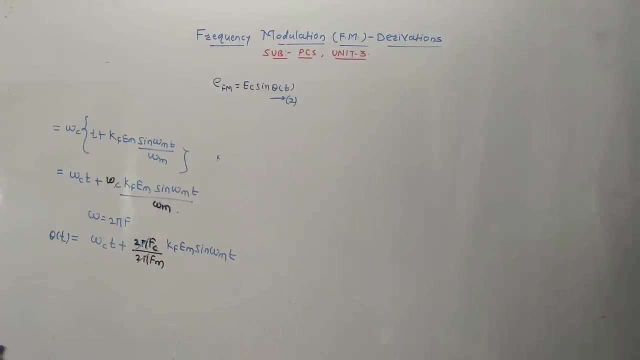 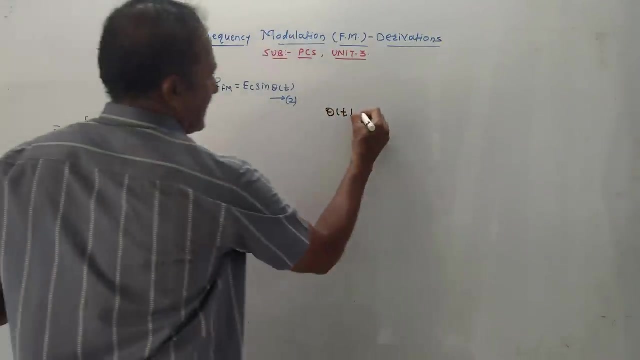 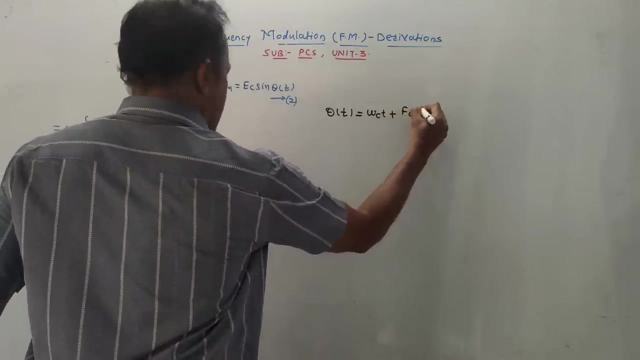 KF, EM sin omega MT. Now I will write the simplified equation Over here. So theta T will be equals to This 2 pi. 2 pi gets cancelled First term, as it is Omega CT plus FC, KF, FM, EM. 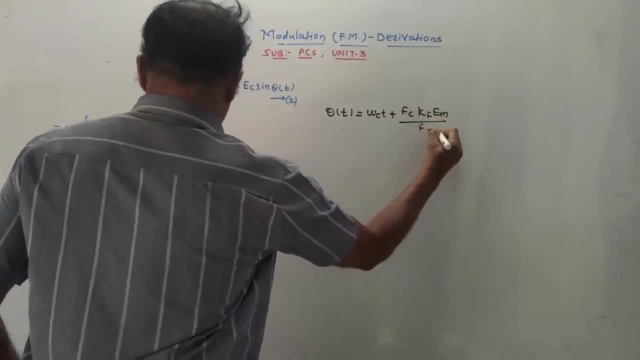 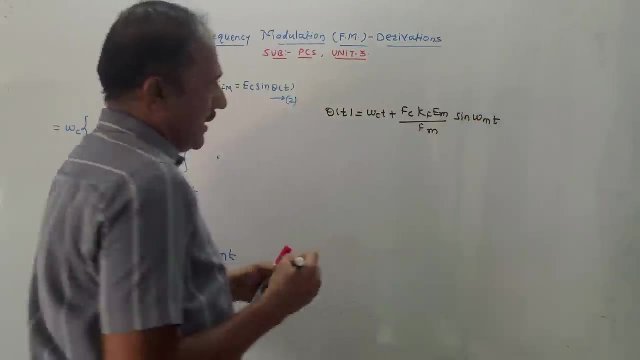 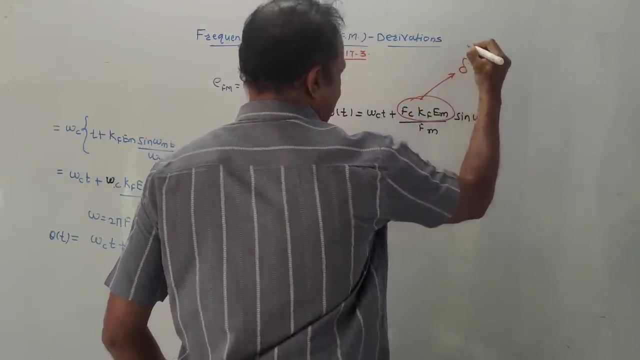 FC, KF, EM upon FM. These terms I have kept it as it is Into sin of omega MT. Now this term FC KF, FM is the equation for delta. Delta is the frequency deviation, So let us replace this value. 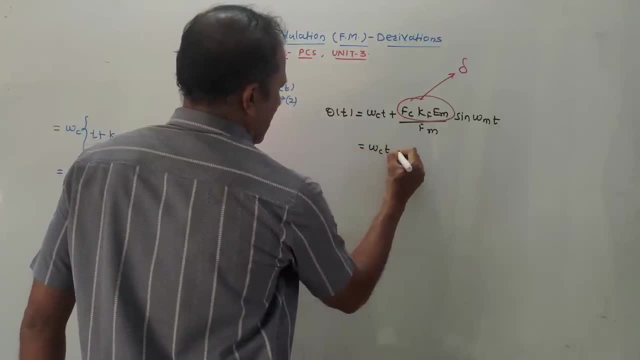 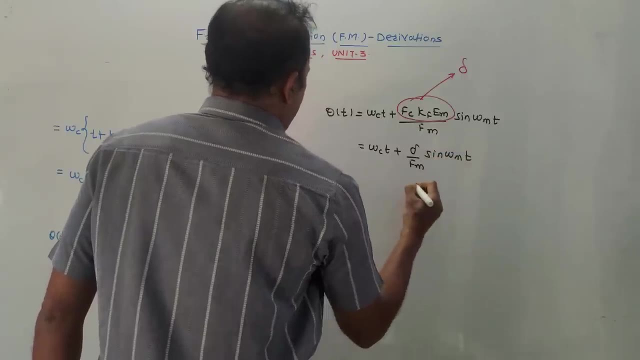 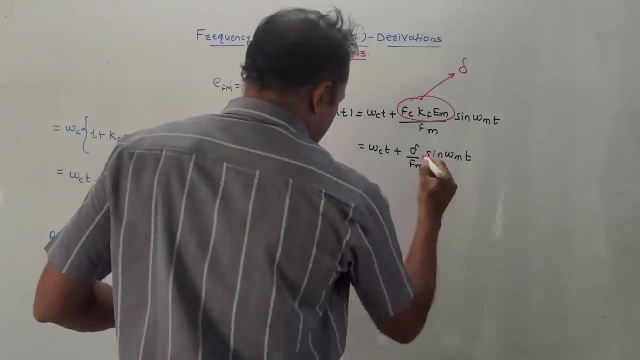 So it can be written as omega CT plus delta upon FM, sin omega MT. Now remember one more equation. Just now we discussed delta upon FM. This ratio Is denoted by MF Or beta. Let us use the notation MF. 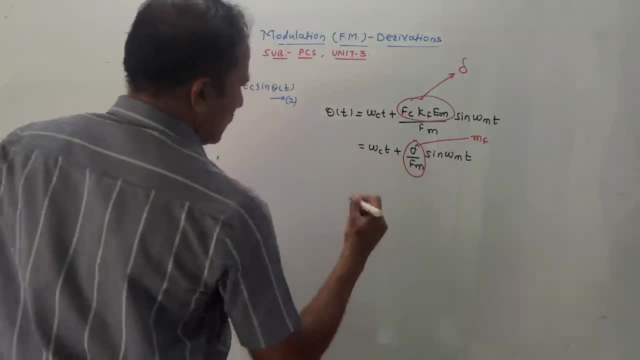 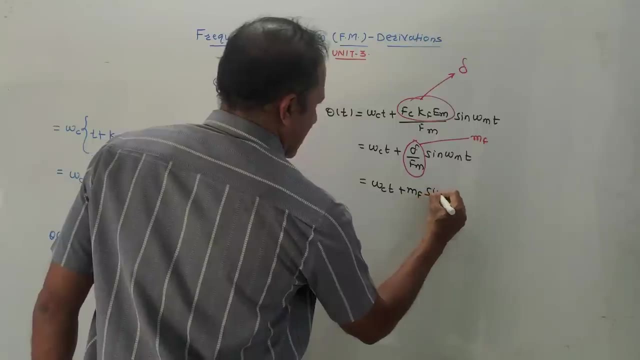 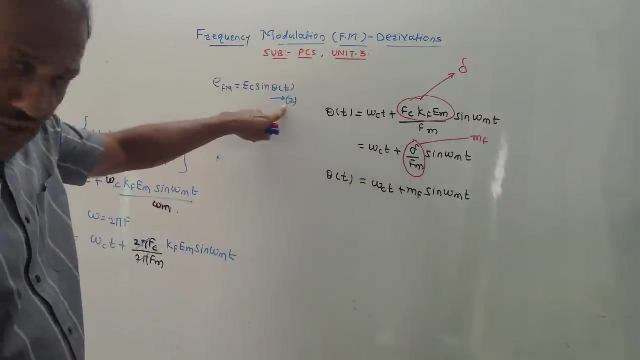 That is modulation index. So put this value, So it becomes omega CT plus MF, sin omega MT. This is the equation of theta T. Put the value of theta T in equation 2. Which we have earlier discussed, So final equation will be EFM. 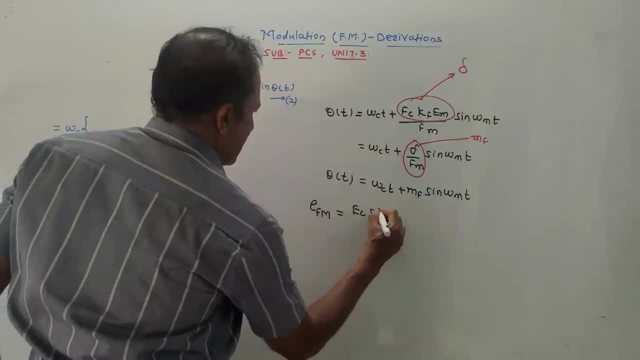 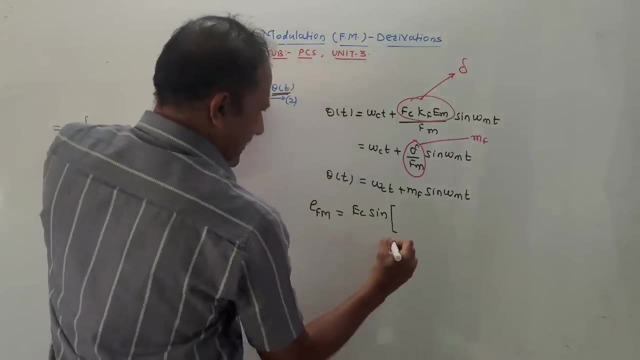 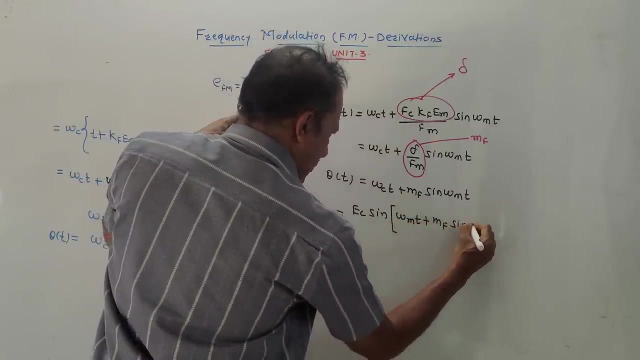 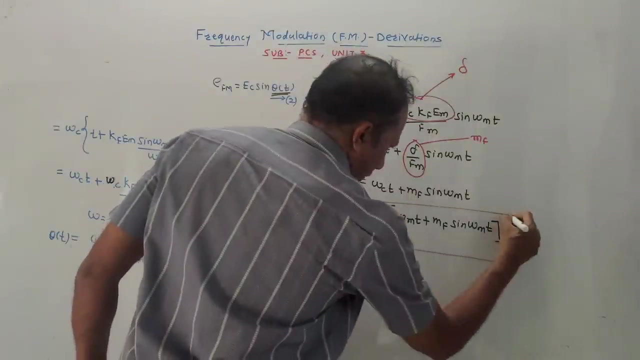 Which is equals to EC sin of this. I am putting value of theta T in equation 2.. So I have kept this same term as it is. Theta T is omega MT plus MF sin omega MT. This is the final equation of 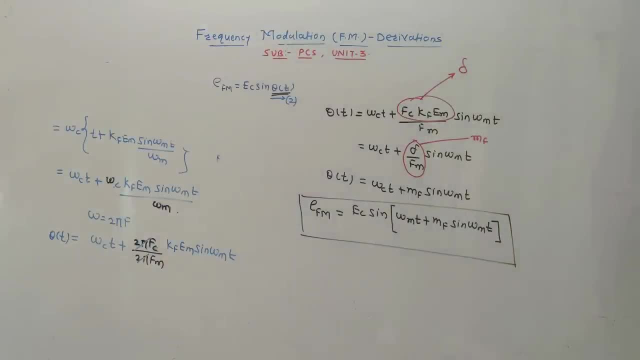 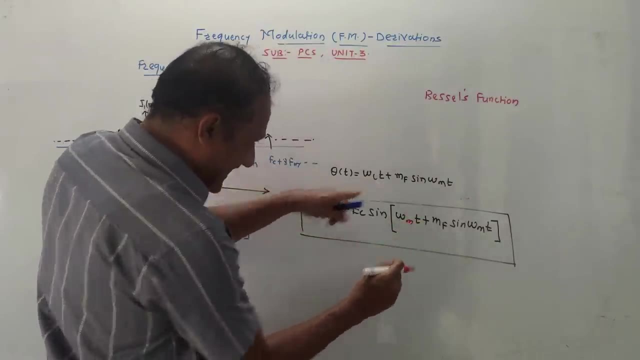 EFM modulated wave. Here there is a small correction Here: omega, As I had written, omega M earlier. Actually this is the first term, omega CT, So this should be omega CT. Rest as it is, Okay. 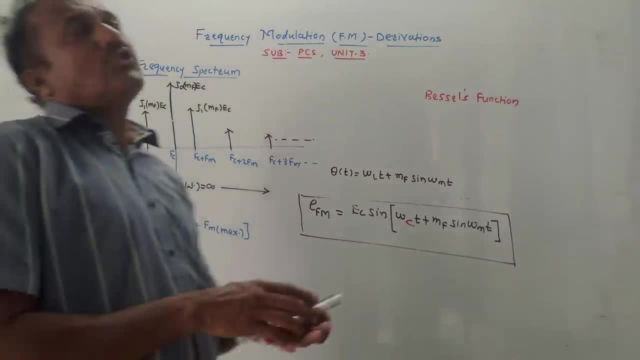 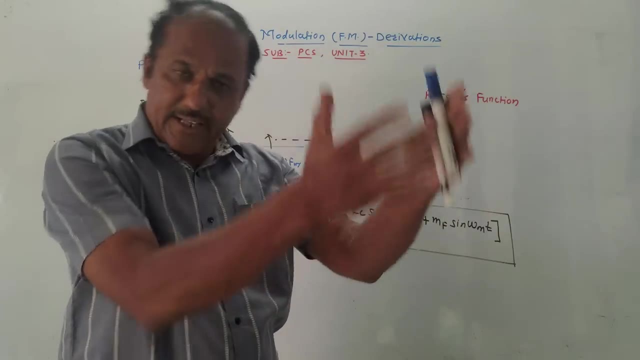 Now frequency spectrum. As you can see, In case of AM wave We had brought a spectrum In that a carrier signal was shown, And at LHS we had lower sideband, At RHS we had upper sideband. 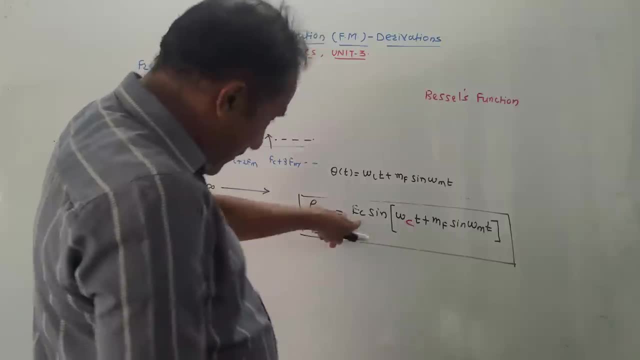 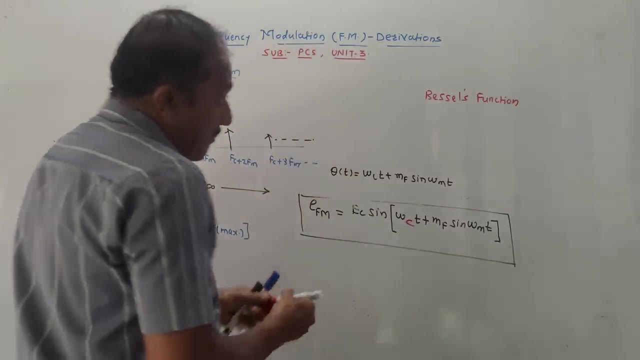 Likewise in this. observe this equation: In this there is a sign of. There is also a sign with it. So we cannot solve it with normal method. For that we have to use Bessel's function. Actually, there is no need to do this in detail. 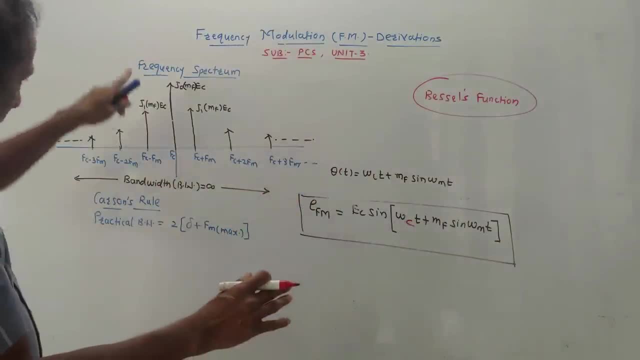 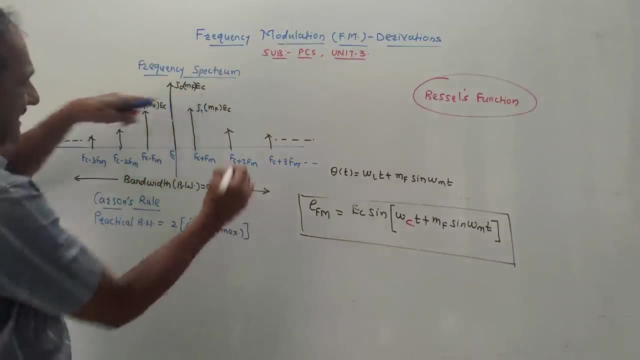 Keep this in mind. In case of FM modulation, The frequency spectrum is: There is a carrier frequency in the middle. Its value is written as J0MFEC. This is it, J0MFEC. J0 is called Bessel's coefficient. 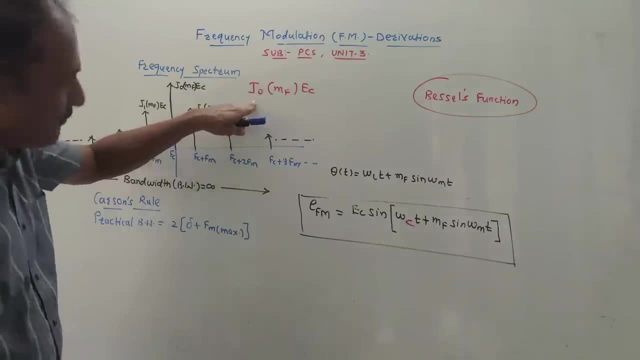 For the 0th term. Both sides of it are sidebands. Likewise there are infinity number of sidebands. The first sideband In RHS, That is Fc plus Fm. Second sideband, Fc plus 2Fm. 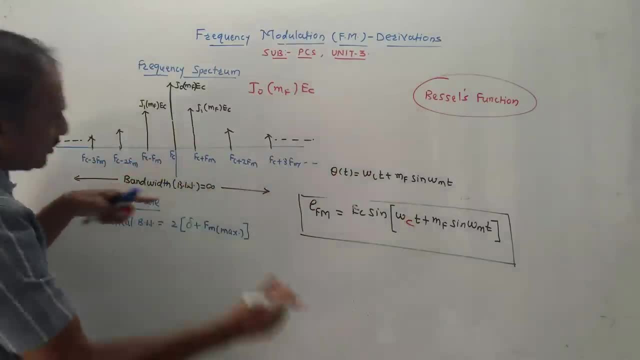 Third sideband, Fc plus 3Fm, And amplitude of sideband Goes on reducing till infinity. Same way In LHS also, We will get infinity sidebands: Fc minus Fm, Fc minus 2Fm. 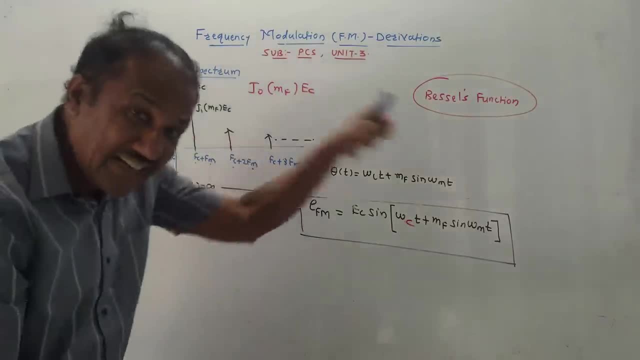 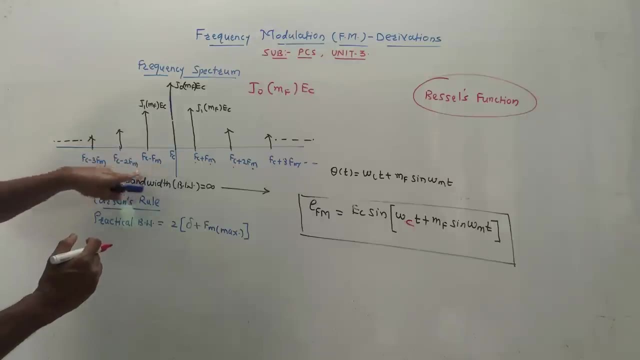 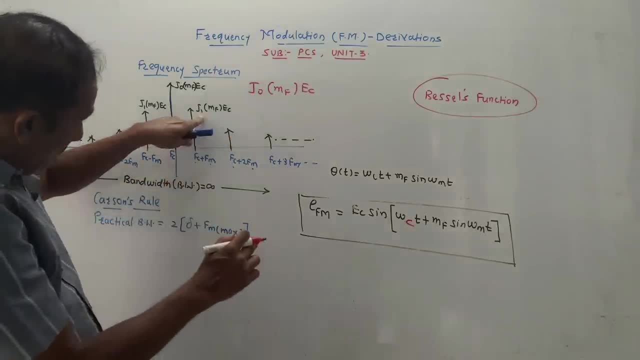 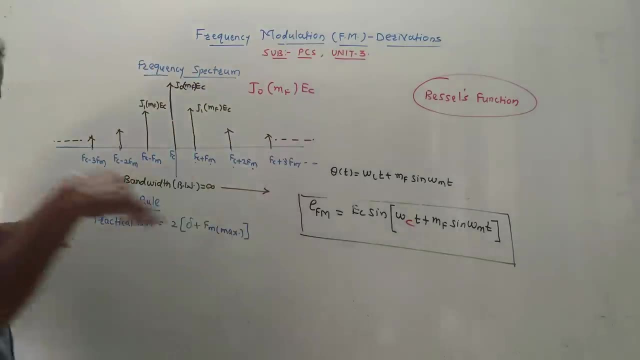 Fc minus 3Fm And so on, The value written here J into Jsupx1MFEC. This Jsupx1. Is again A Bessel's function Likewise. So I say You have to keep in mind. 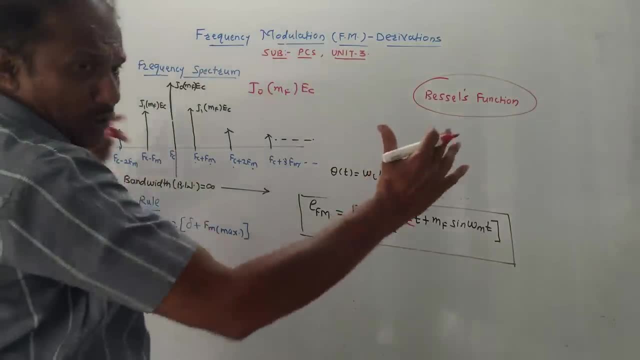 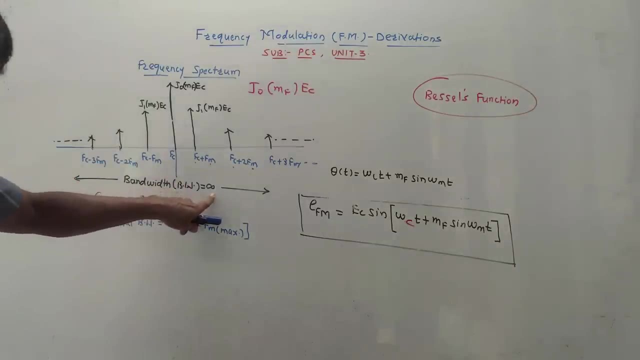 In FM wave You will be Ideally getting Infinity number of Upper sidebands And infinity number of Lower sidebands. So ideal bandwidth Of FM wave Is infinity. But Practically This bandwidth Is calculated. 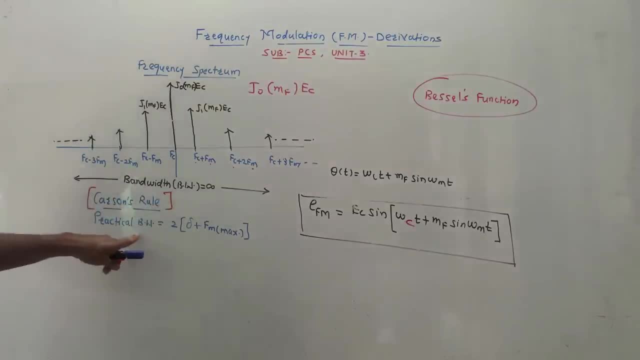 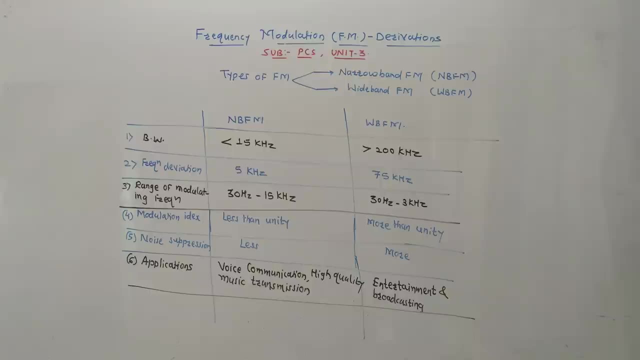 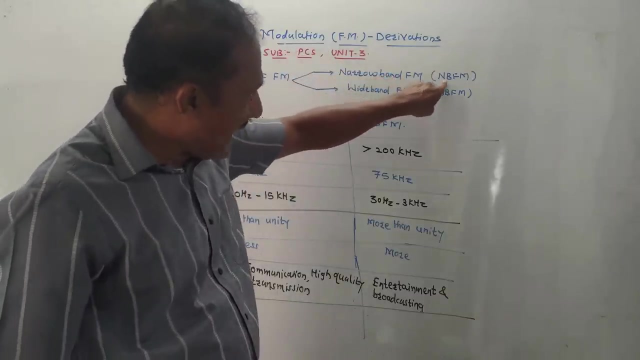 Using Carlson's rule. This rule is Practically Calculated. band width is 2 in the bracket delta plus FM max. the next part is types of FM. there are usually two types of FM. first is narrow band FM and BFM. second is 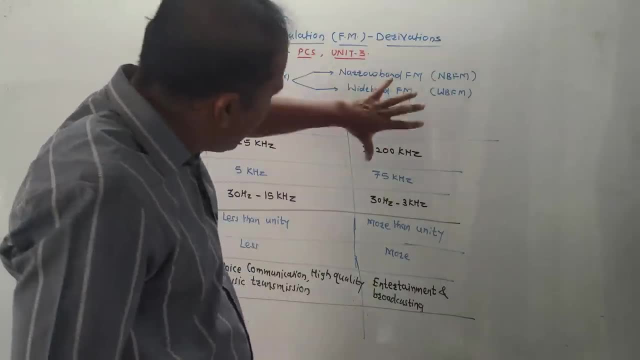 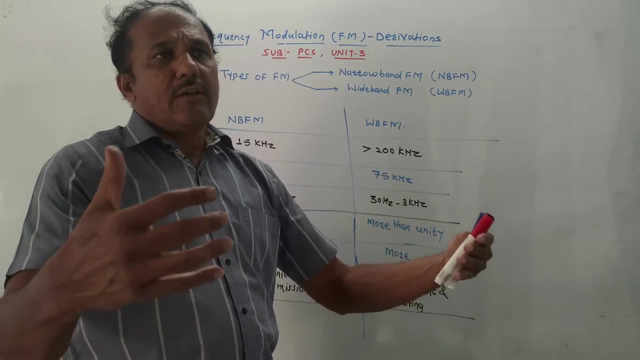 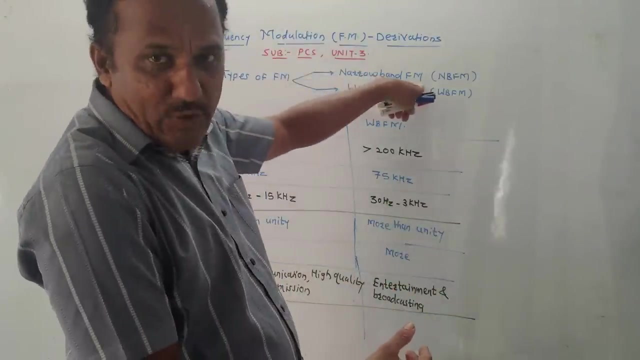 wideband FM, WBFM. now why these types are there? just a deco, I may learn kiki, ideally bandwidth infinity with it, but there are certain restrictions in practical cases. so practical restriction Honecki were just say: have look, narrow band FM use curving in many cases, whereas in some cases 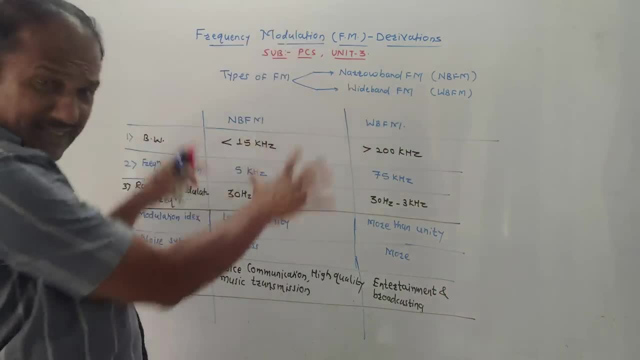 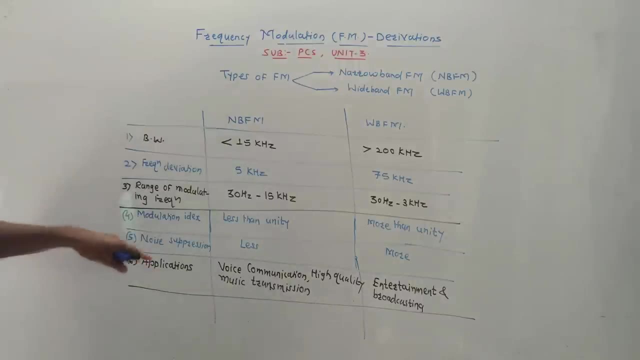 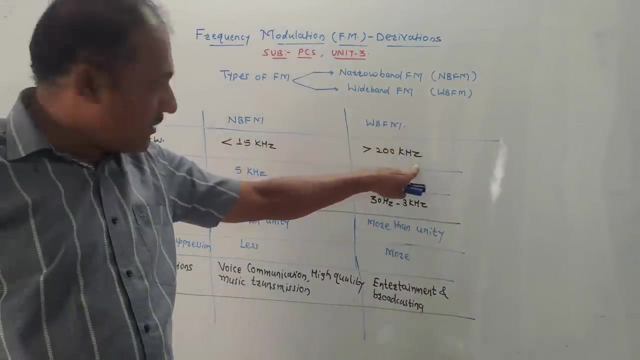 wideband FM is prepared from the example of you. comparison is asked, so compare narrowband FM and wideband FM. so I have made a list of comparison points. so first is bandwidth: for NBFM is less than 15 Hertz. for WBFM it is greater than 200. 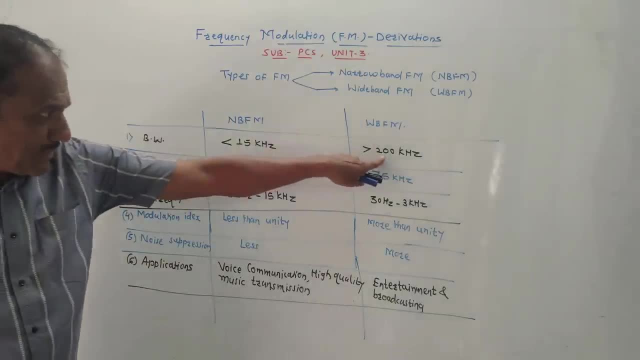 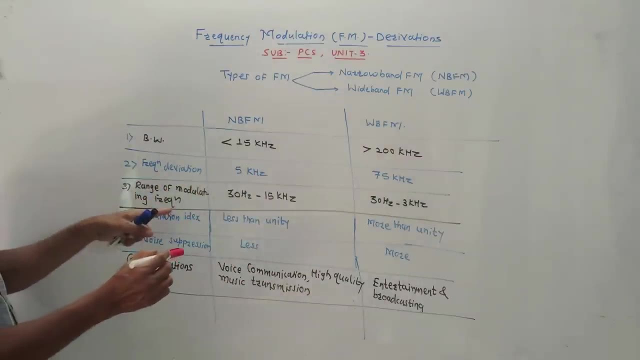 kilohertz, it is less than 15 kilohertz. and second WBFM, it is greater than 200 kilohertz. frequency deviation: 5 kilohertz. in this case it is 75 kilohertz. range of modulating frequency is 30 Hertz. 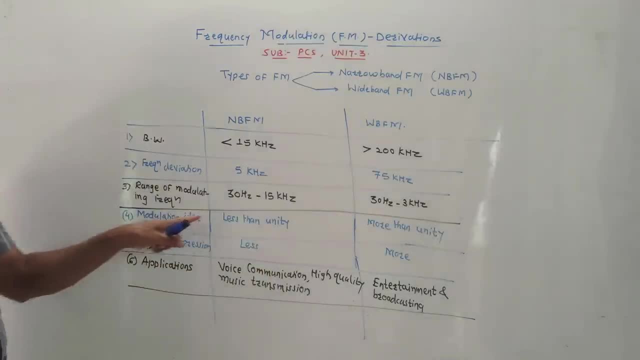 to 15 kilohertz, 30 Hertz to 3 kilohertz, then modulation index is less than 1. that is less than unity. in second case, it is more than unity. NBFM is less responsible for less noise suppression and it gives more noise suppression and 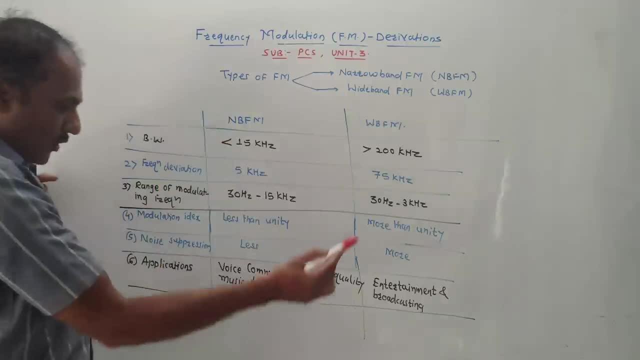 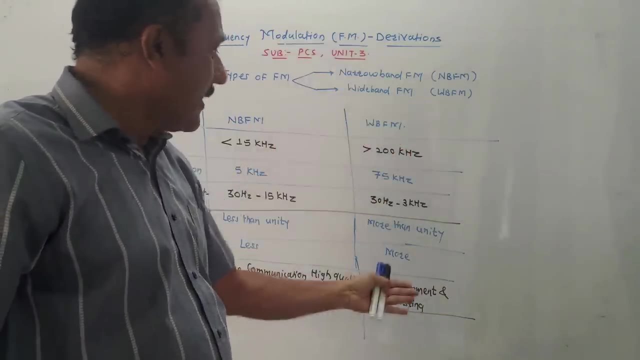 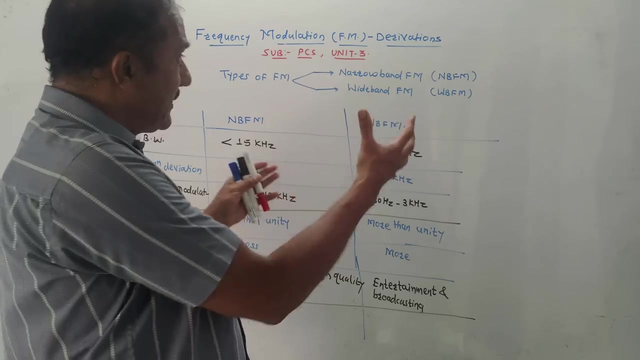 applications. voice communication, then. for high quality of music transmission, NBFM is used, whereas in case of wireless systems, WBFM is used, or it is used in entertainment and broadcasting applications. so, dear students, that's it for today's session. we have covered the derivation and theoretical part related to frequency modulation. in the next 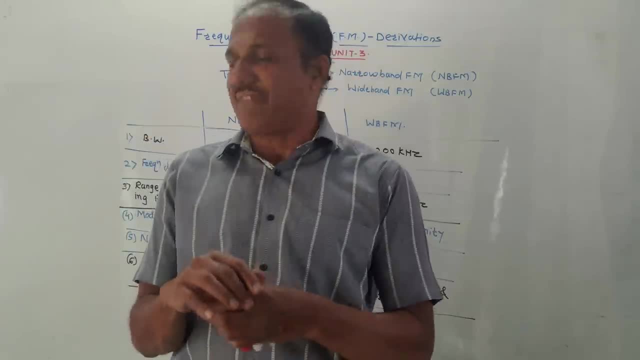 session will solve numericals related to FM. so thank you, thanks a lot.